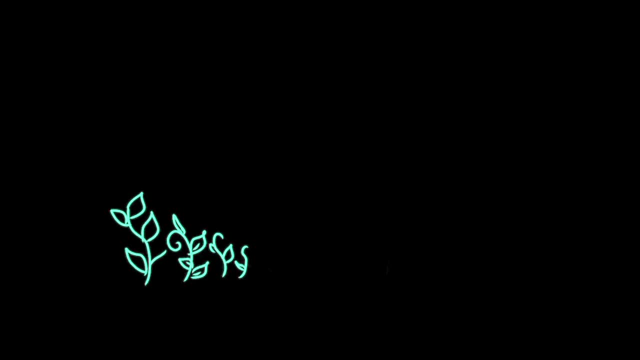 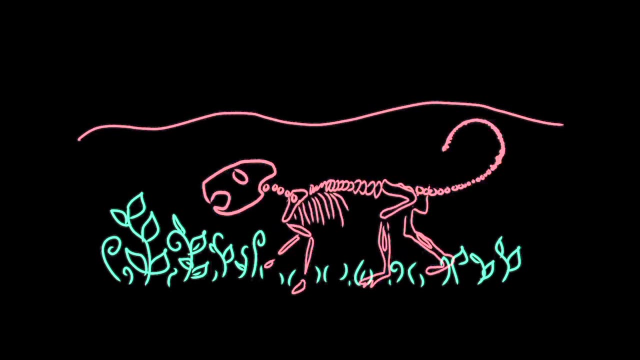 formed in the geologic past from the remains of ancient organisms. Plants and animals that died millions of years ago became buried in the soil, partially decomposed and were exposed to a chemical re-arrangement of the energy contained within their bodies into the fossil fuels we use. 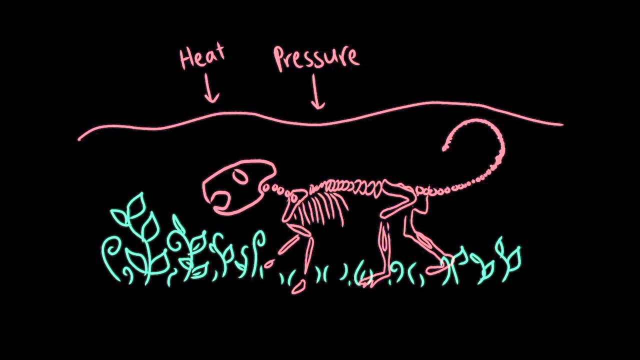 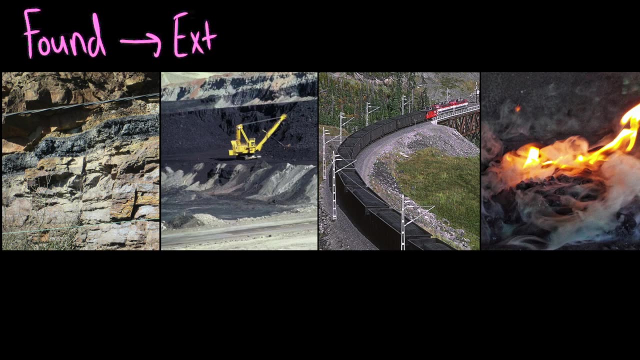 today Because they take so long to form. we have a finite amount of non-renewable resources in the earth right now. The lifespan for fossil fuels is a broken loop, a one-way ticket: First the fossil fuel is found, Then it has to be extracted. Extracting fossil fuels can involve destructive 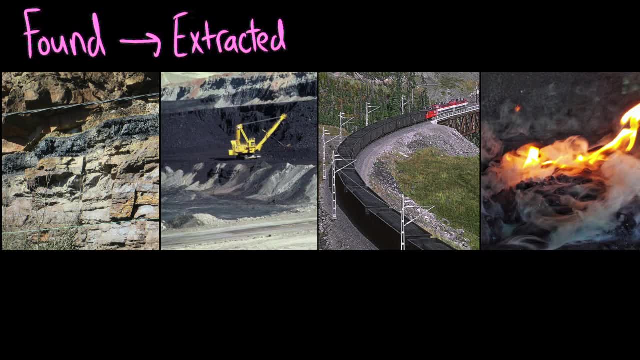 mining processes that can pollute surrounding habitats. Then it has to be transported to wherever it will be used, And using fossil fuels means burning them, which releases greenhouse gases and other pollutants into the atmosphere. Also, it can take energy to refine and process some types of fossil fuels so that they're more helpful to us like 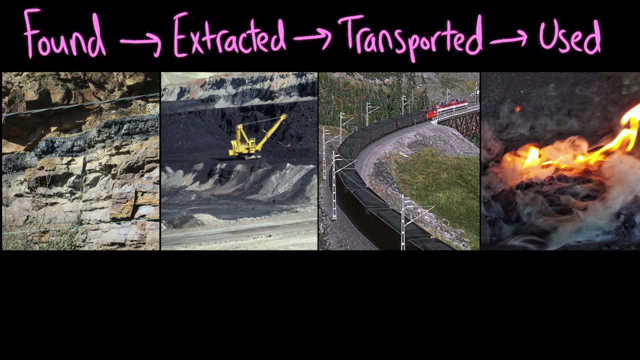 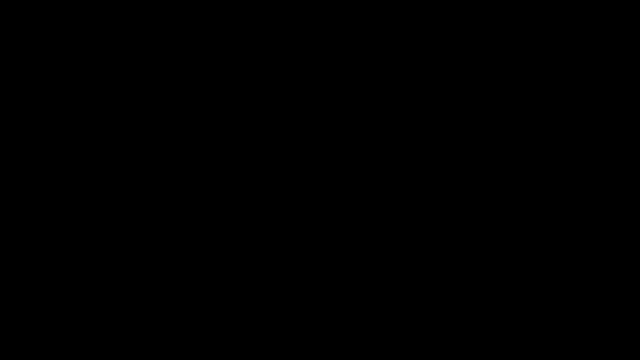 turning crude oil into petroleum gas, diesel and jet fuel And burning the fossil fuels transforms that energy into a less organized form of energy like heat and ash. Not all fossil fuels are the same, And this is because different kinds of organic material were heated and compressed in. 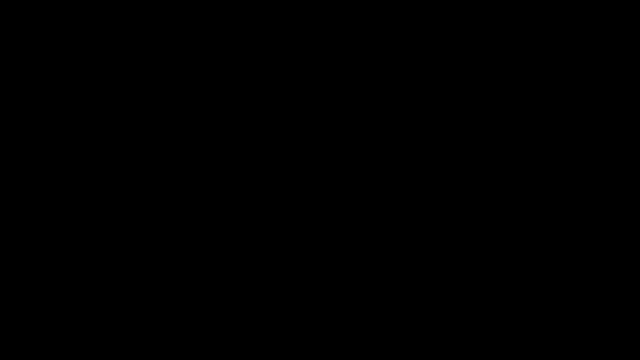 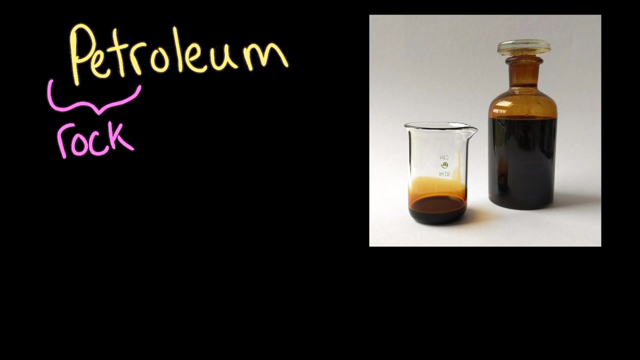 different ways, creating different kinds of fossil fuels. One of these kinds of fossil fuels is petroleum. The word petroleum comes from the latin word for rock, petra, and the latin word for oil, oleum. This makes sense because it's an oily substance that's found in reservoirs, trapped in. 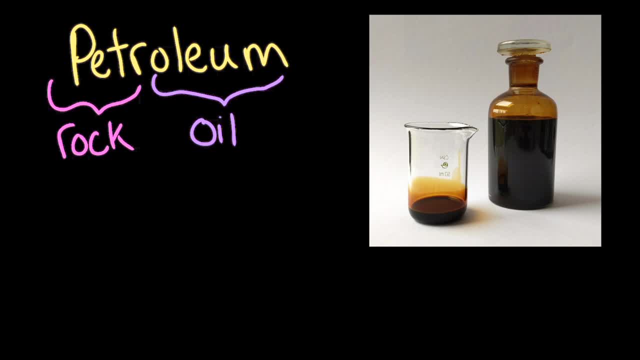 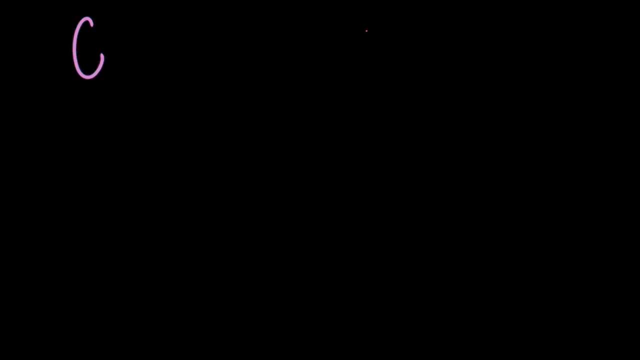 rock. Humans have been using oil for a very long time. Early civilizations found it bubbling up from the ground at natural levels. This is because the oil is so rich that it can be used as a fuel. The oil they saw coming straight out of the earth is called crude oil or crude petroleum. 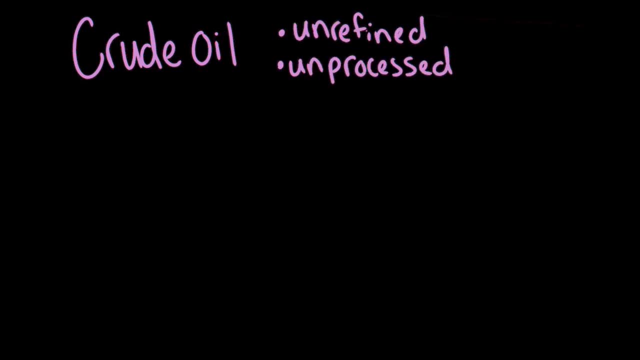 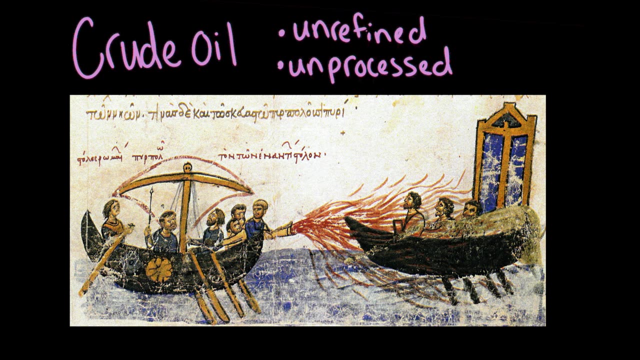 which means that it is unrefined and unprocessed. Crude oil was probably one of the ingredients in Greek fire, which was a flamethrowing weapon that the Byzantines would fling at their enemies. Today we refine crude oil into many products like gasoline and diesel for vehicles, kerosene for 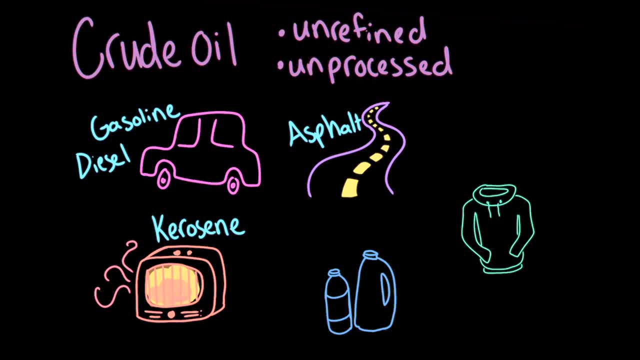 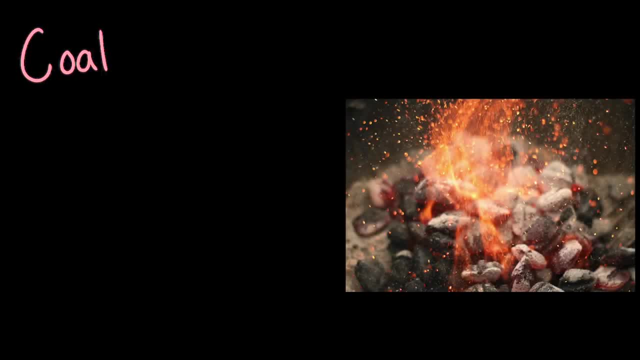 heating and asphalt for road construction. It's also used to make plastics and synthetic fabrics. Another type of fossil fuel is coal, which we mostly burn to make electricity, but it can also be used for heating and cooking. It's a solid, shiny, black, flammable rock. 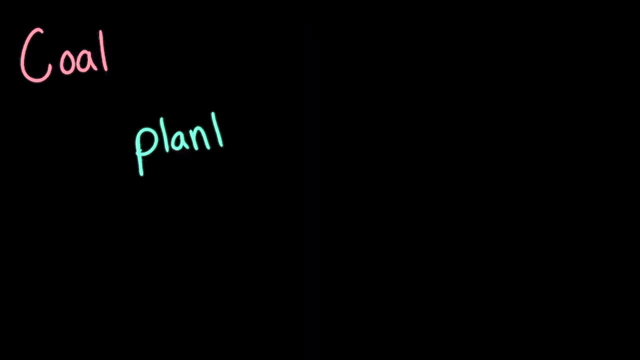 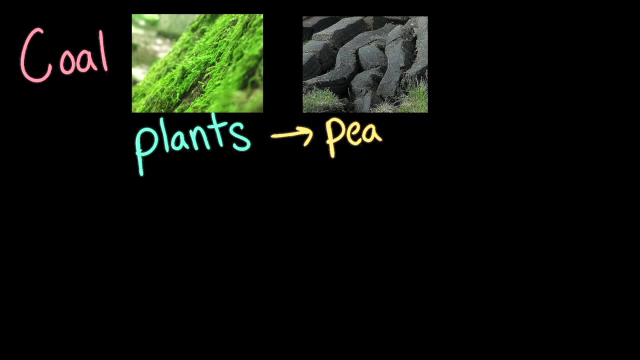 which is mostly formed from the carbon remains of fossilized plants like moss. Over thousands of years, plant material transforms into a carbon rich compound called peat, and then, with some pressure, it becomes soft coal, which is called lignite, and then, with more pressure, 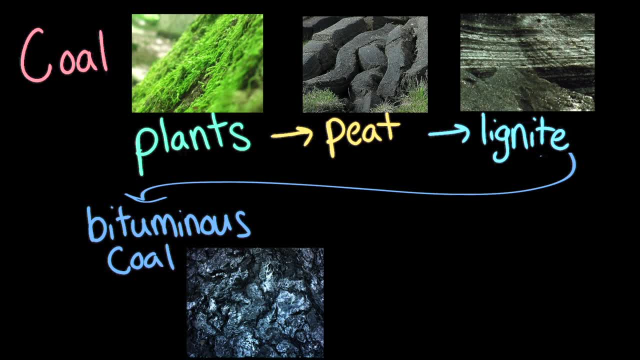 it becomes bituminous coal And then finally it becomes a hard coal called anthracite. The longer the plant remains are put under pressure, the more energy dense it becomes. So if you burned anthracite you would get a lot more energy than if you burned peat. Burning coal releases carbon. 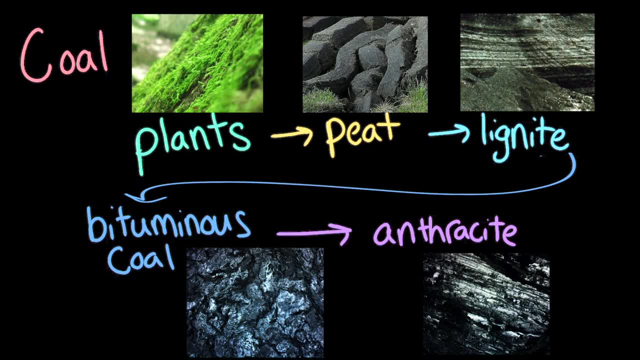 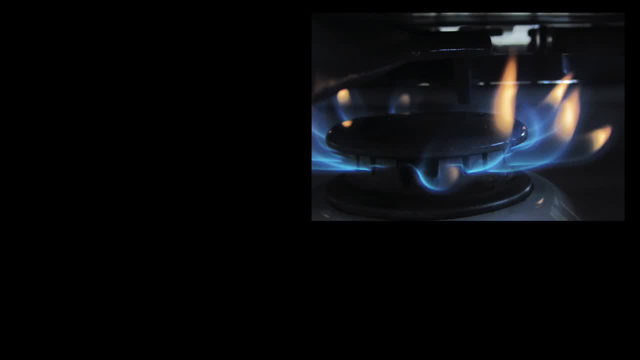 dioxide, sulfur dioxide, nitrogen oxides and other gases into the air. So coal is one of the dirtiest fossil fuels. The cleanest burning fossil fuel is natural gas, meaning that it emits the least amount of carbon dioxide or other air pollutants. This is not the same type of gas as we put into. 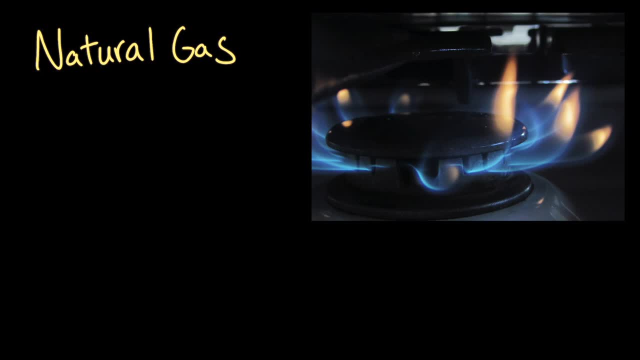 our vehicles. That type comes from petroleum. Instead, natural gas is mostly used for generating electricity, heating homes and cooking food. Your oven, furnace, water heater, dryer or grill- all might run on natural gas. Natural gas is a naturally occurring mixture of gases. 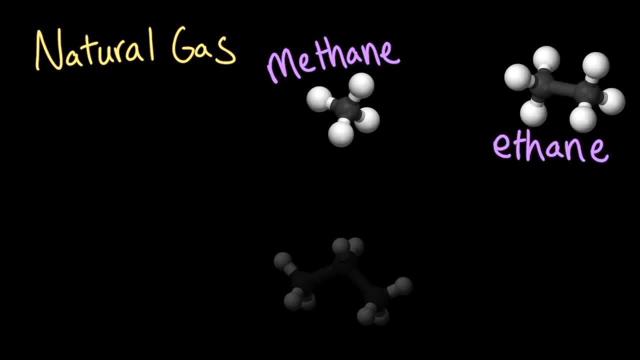 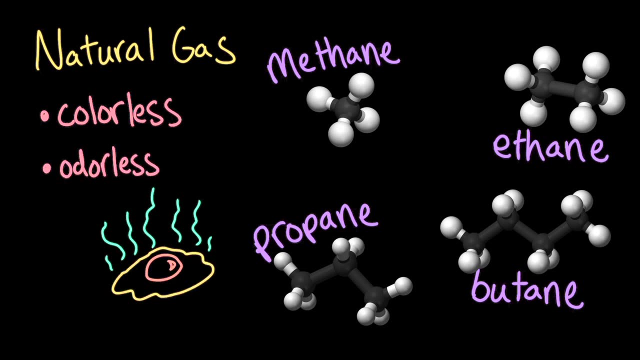 And it's mostly made up of methane, ethane, propane and butane. The gas is colorless and odorless, so natural gas companies often add a rotten egg smell to the fuel to make leaks easier to detect. But even though we can't see or smell natural gas, humans have been detecting it and using it. 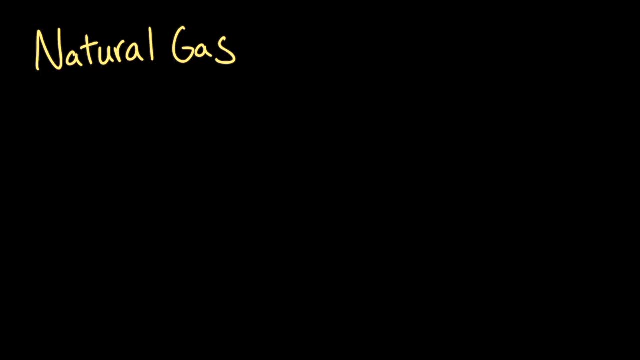 for centuries. There is evidence that more than 2,000 years ago, people in China created bamboo pipelines to transport the gas so that they could use it to boil salt water to separate out the salt, And today we still use pipelines to transport gas across land. 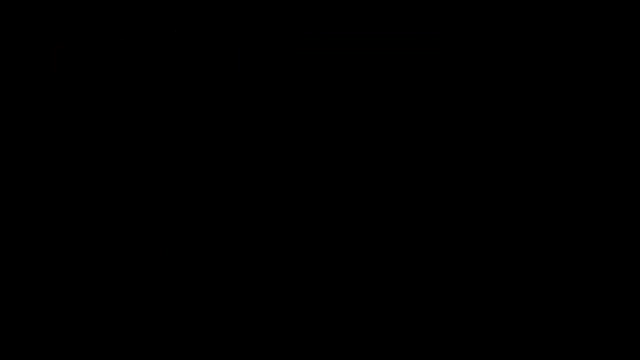 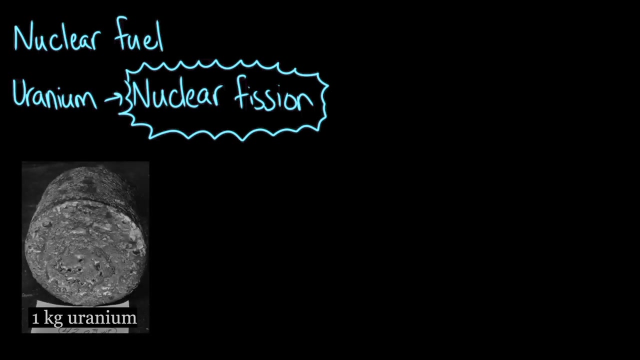 although they're no longer made out of bamboo. Another kind of non-renewable resource is nuclear fuel. Nuclear power plants don't burn fossil fuels. Instead, they split uranium through something called nuclear fission. Just 1 kilogram of uranium can produce 24 million kilowatt hours of energy. 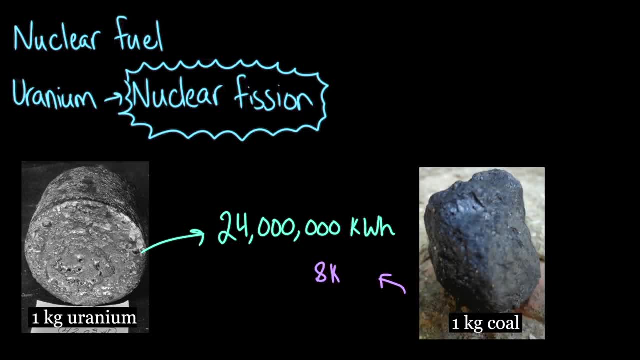 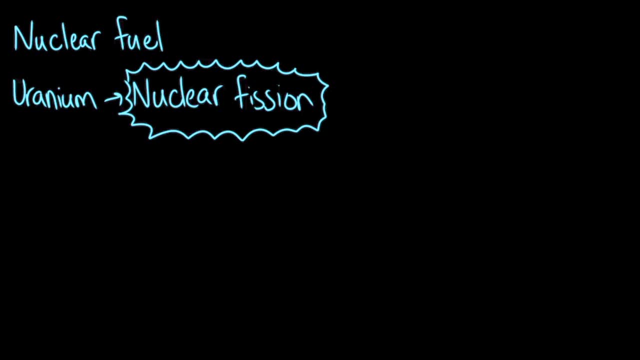 Compare that with 1 kilogram of coal, Which can produce 8 kilowatt hours of energy. In other words, nuclear fission produces a lot of energy. It also produces a lot of heat, which we mostly use to make electricity.